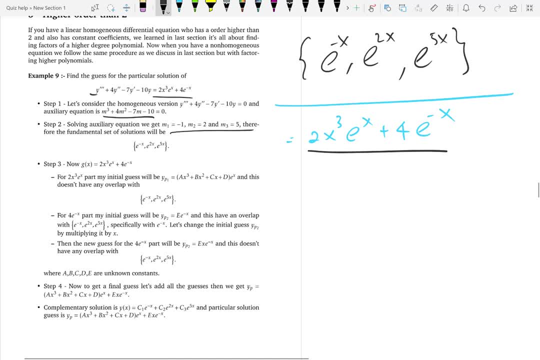 if you look at this gx, let's write the initial guess for the particular solution. So we have a cubic function, time exponential function. So the cubic function is written: x, cube plus bx, square plus cx plus d, right? Yes, times e to the x Plus. now we use the superposition approach, right? 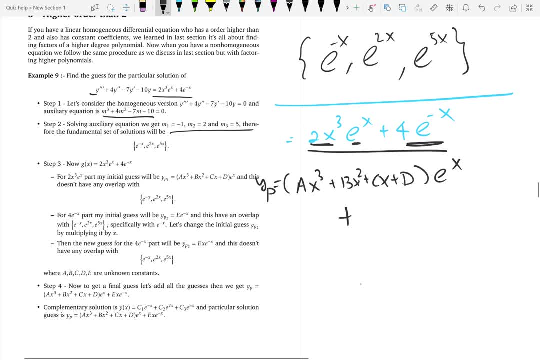 Constant times e to the negative x. So d e e times e to the negative x. So this is my initial guess. Good, Now do we have overlap: e to the negative x? Yes, we have an overlap, But e to the 2x and e to the 5x is not here. So how do we handle the overlap? 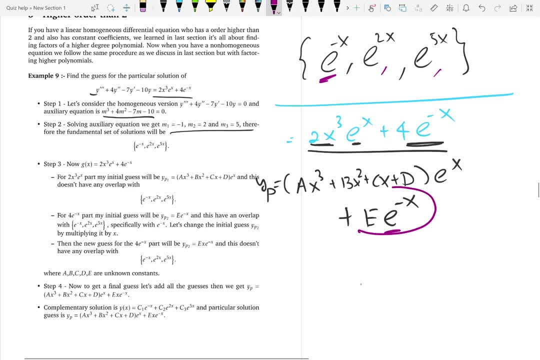 of e to the negative x. This is the offended party, right? We just multiply the offended party by x. So just multiply e by x, So it's e to the x. Do not multiply the whole thing, Okay, unless the whole thing is offended, unless the whole thing is. 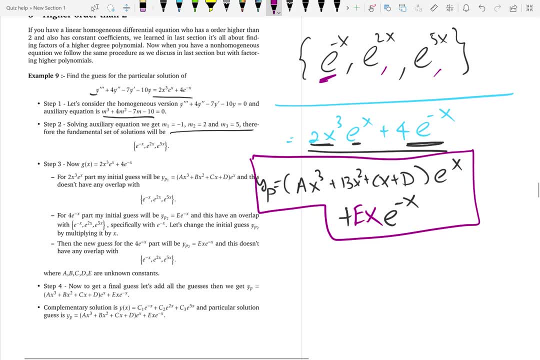 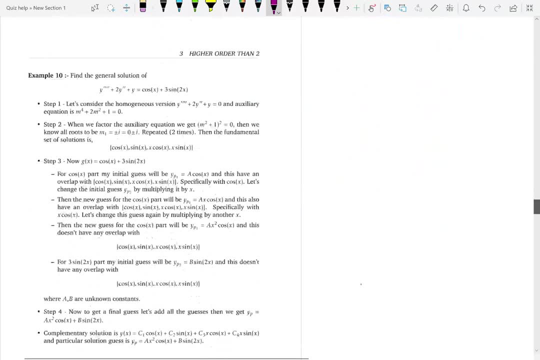 overlap. So this is the guess for the particular solution. So it's really the same process. okay, it's just you have more functions on the fundamental set of solution. Okay, let's look at one more example, because we can, of course, learn something new. So here we have a third. 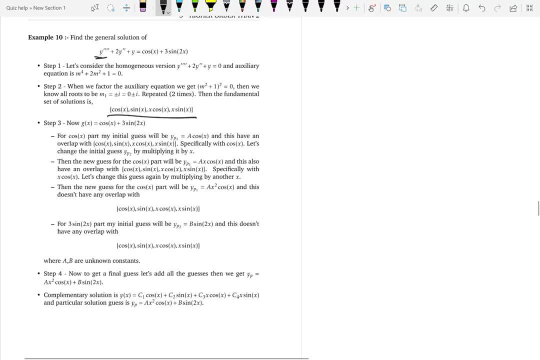 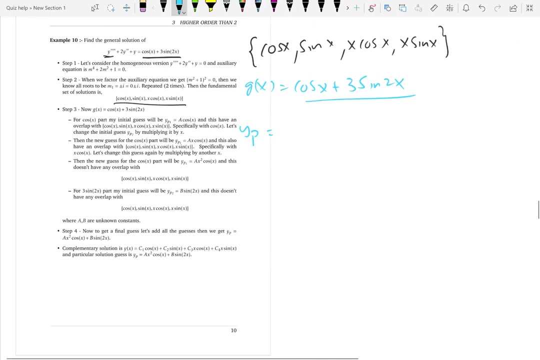 fourth order differential equation, and they have given the fundamental set of solution as cosine x sine x x. cosine x x sine x. okay, all right. and the right hand side is gx. is cosine x plus 3 sine 2x. Okay, how do you write the initial guess? Well, the initial guess would be a cosine x. 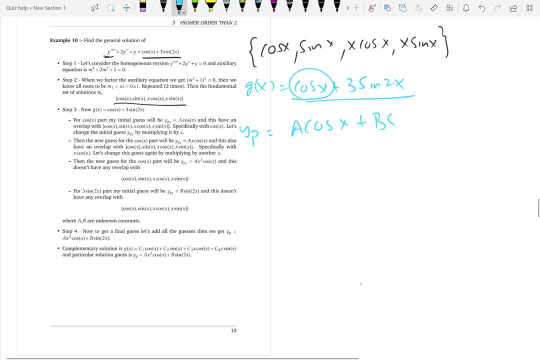 this is for this. cosine x, part right. a cosine x plus b. sine x plus. here for sine 2x plus part c: sine 2x plus d, cosine 2x right. Okay, that's the initial case. Now do we have an overlap? Well, cosine x. 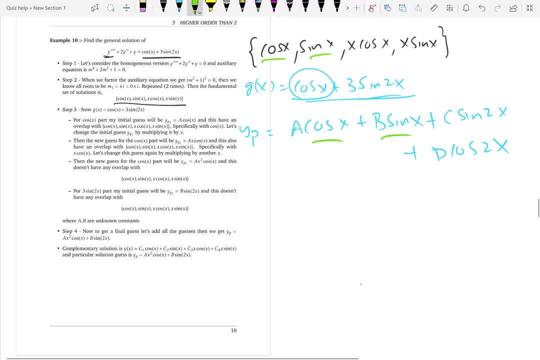 cosine x overlap sine x sine x overlap x cosine x. no, so there's no. you don't have x cosine x here, so we do not have overlap in these parts, right? Okay, so these are the two offended parties. so we multiply them by x, so ax cosine x plus bx sine x. don't multiply these by x c sine 2x. they are just.